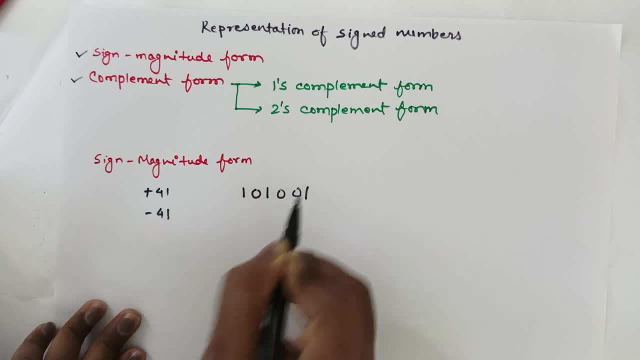 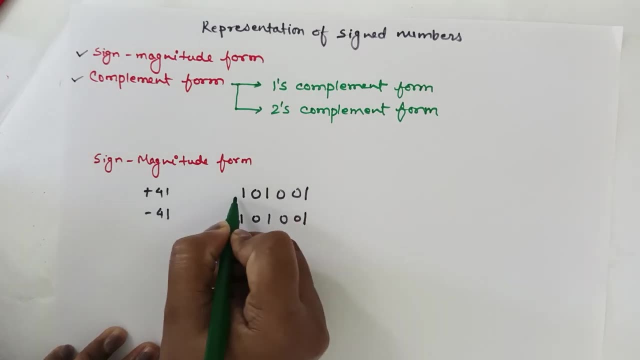 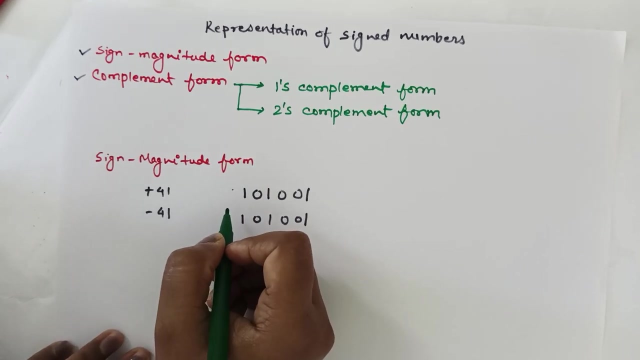 1 0, 1, 0, 0, 1.. 1 0, 1, 0, 0, 1.. We simply add one extra bit here in front of this number for the representation of the sign: For positive we add 0 and for negative we add 1.. So this: 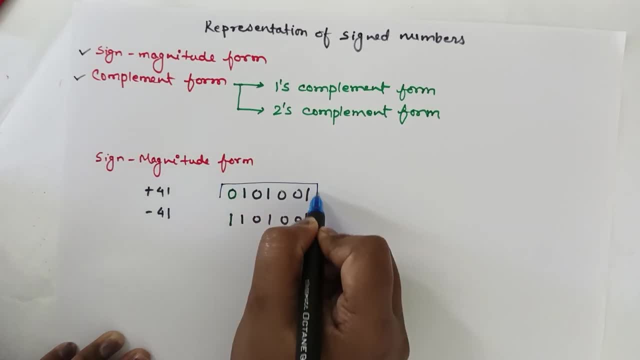 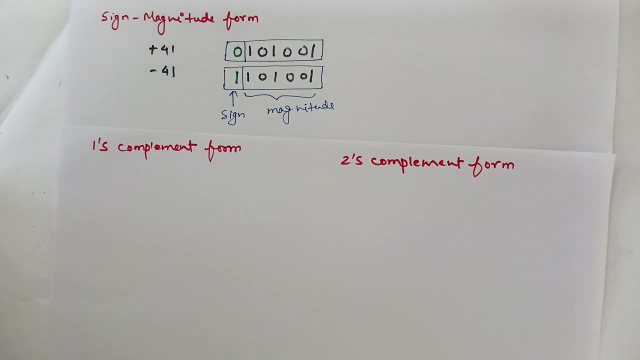 is how we represent it: signed numbers. So this will be positive 41 and this will be negative 41.. This is magnitude. This will be positive 41.. And this is sign. Let's start one's complement form. You'll take the same example For plus 41 in one's complement. it will be same as signed magnitude. 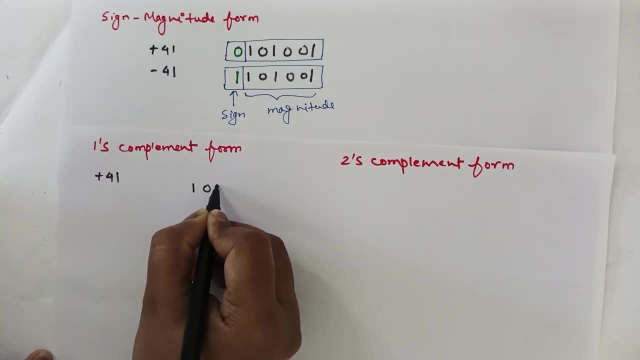 form. So we write the binary equivalent of 41, 1, 0, 1 0, 0, 1.. And we add an extra sign, 0 for plus sign. This is the representation for plus 41 in one's complement. This is sign bit. 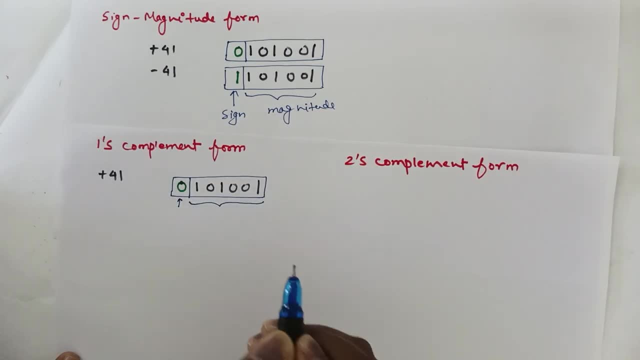 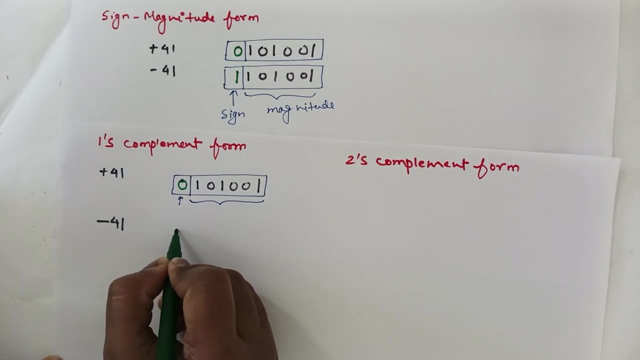 and this is magnitude. How to write minus 41 in one's complement form. We take one's complement of this positive 41. We have this: 0, 1, 0, 1, 0, 0, 1.. This is positive 41 and we will take. 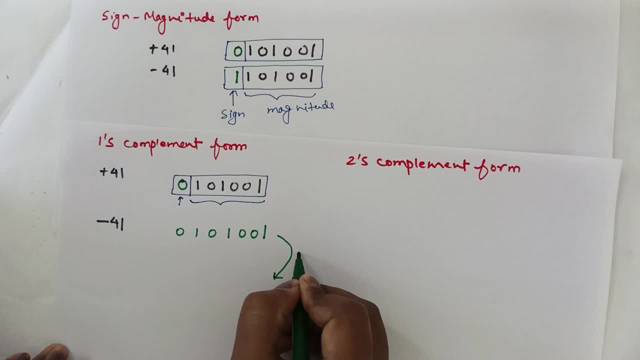 one's complement of this. How to take one's complement? We simply write the opposite numbers for these numbers: 0, 1, 1, 0, 1, 0, 1.. So this will be the representation of negative 41.. This is sign bit and this is. 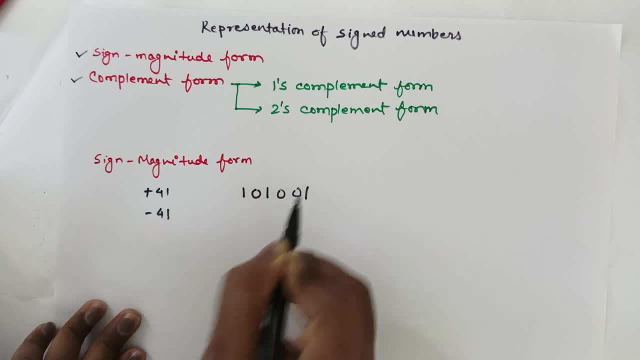 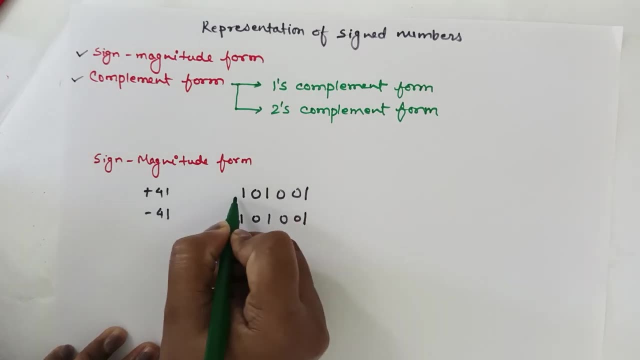 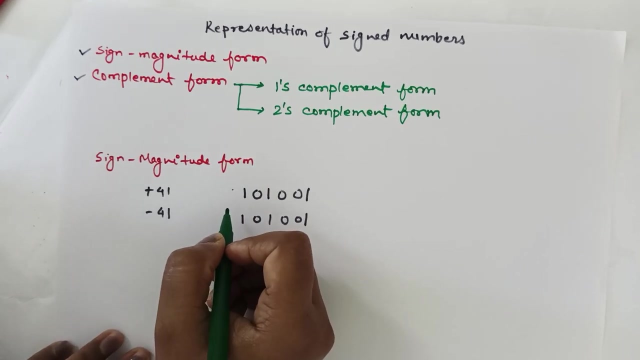 1 0, 1, 0, 0, 1.. 1 0, 1, 0, 0, 1.. We simply add one extra bit here in front of this number for the representation of the sign: For positive we add 0 and for negative we add 1.. So this: 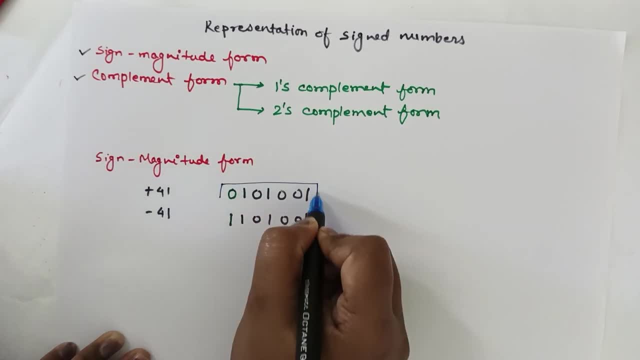 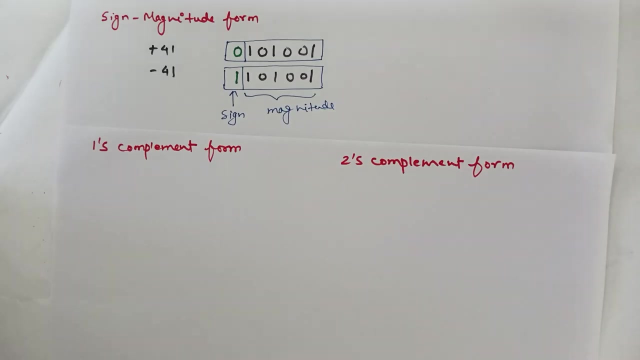 is how we represent it: signed numbers. So this will be positive 41 and this will be negative 41. This is magnitude, This is sign. Let's start one's complement form. We will take the same example For plus 41 in one's complement. it will be same as signed magnitude form. So we write the binary. 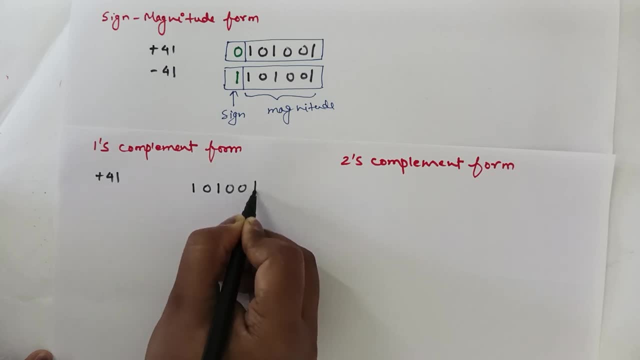 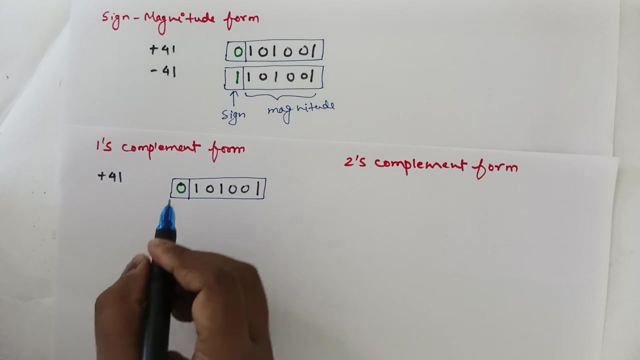 equivalent of 41. 1 0, 1, 0, 0, 1. 0 for plus sign. This is the representation for plus 41 in one's complement. This is sign bit and this is magnitude. How to write minus 41 in one's complement form: We take one's complement. 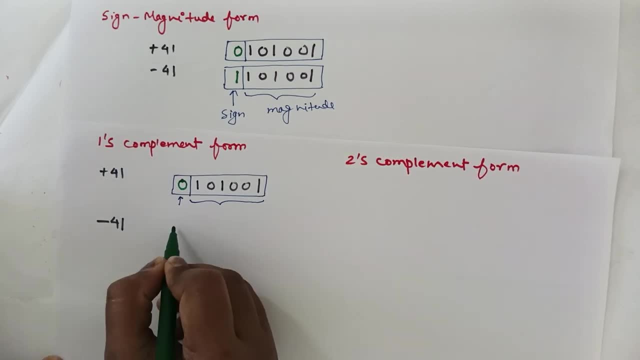 of this positive 41. We have this: 0, 1, 0, 1, 0, 0, 1.. This is positive 41 and we will take one's complement of this. How to take one's complement? We simply write the opposite. 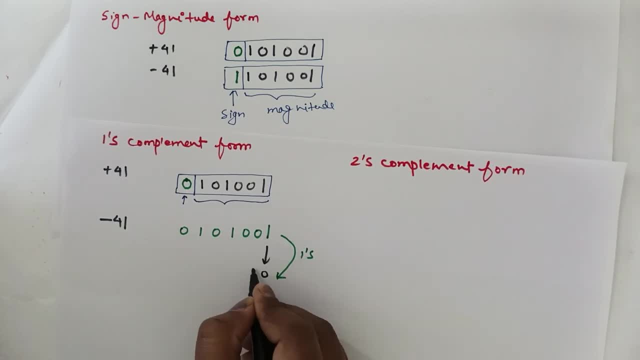 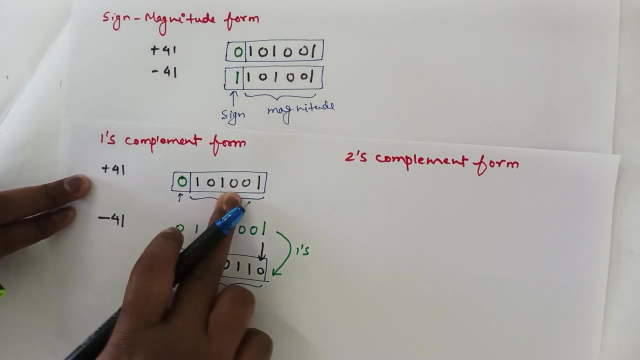 numbers for these numbers: 0, 1, 1, 0, 1, 0, 1.. So this will be the representation of negative 41. This is sign bit and this is magnitude. This is how we represent a number- positive number and negative number- in one's. 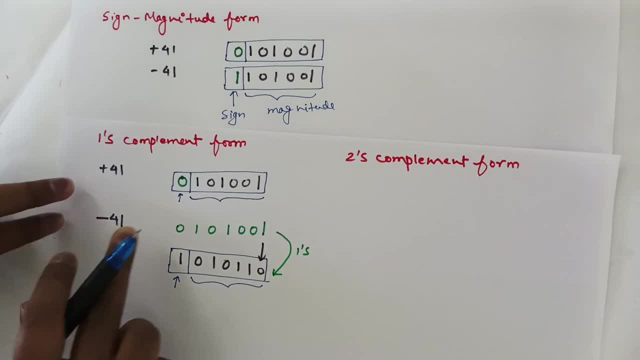 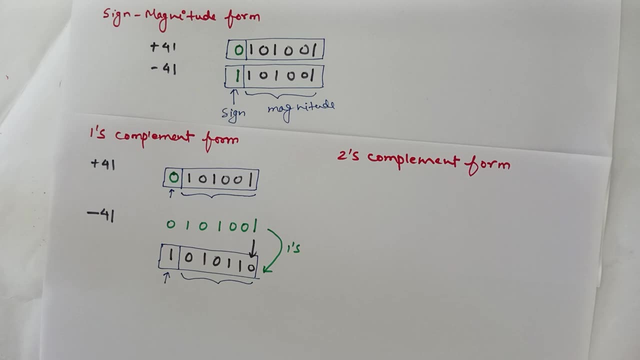 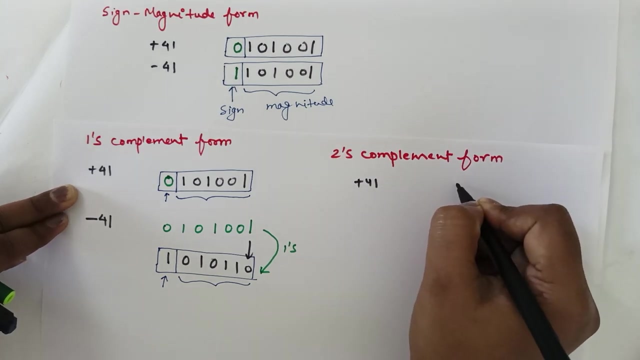 magnitude. This is how we represent a number- positive number and negative number- in one's complement form. Now we will see in two's complement form We see the same example for plus 41. It will be same 1, 0, 1, 0, 0, 1.. We add a sign bit in front of the number, 0, 0, for 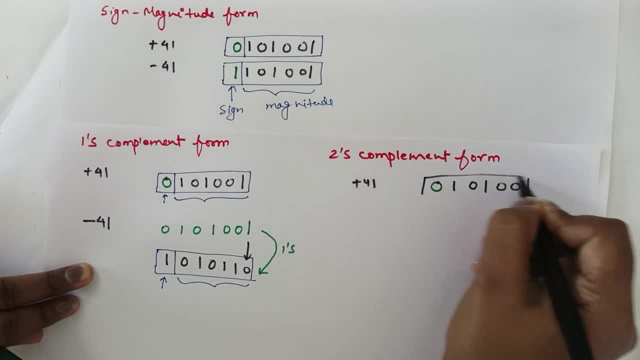 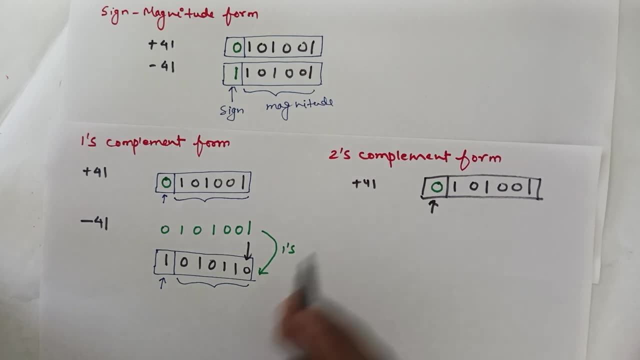 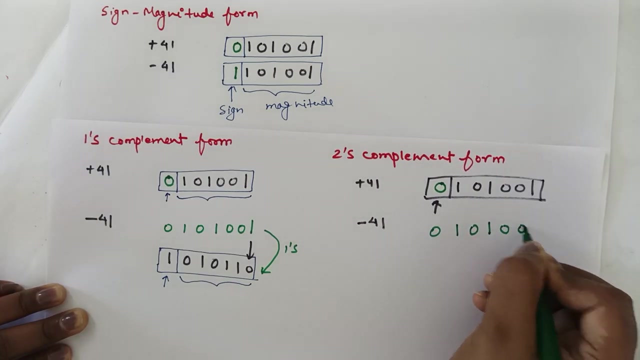 plus sign. This is sign bit, and for minus 41, we find the one's complement plus 1.. That will be minus 41.. Now we will be giving two's complement. This is 0, 1, 0, 1, 0, 0, 1.. First, find one's complement. 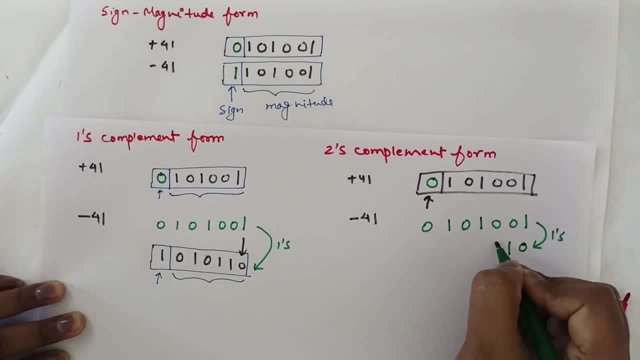 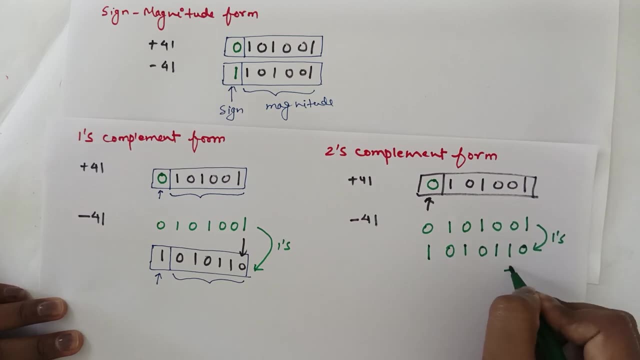 0, 1, 1, 0, 1, 0, 1.. And then plus 1.. So this will give 1, 1, 1, 0, 1, 0, 1.. 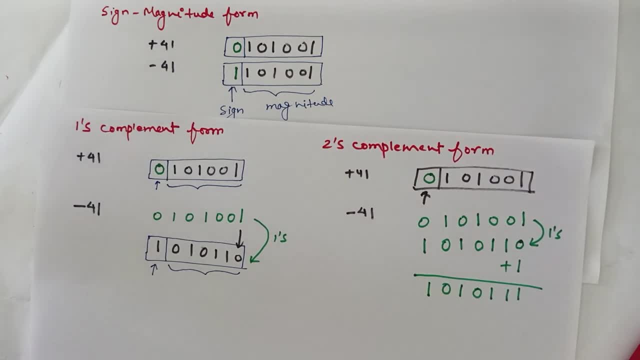 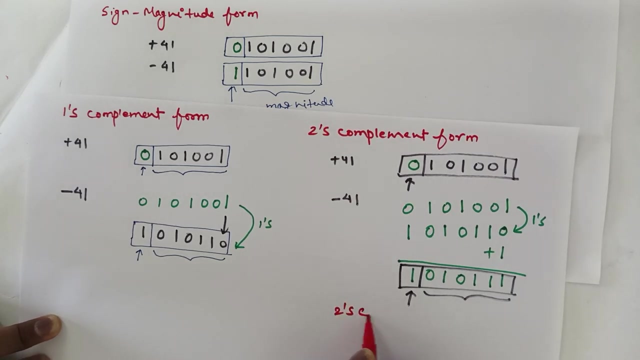 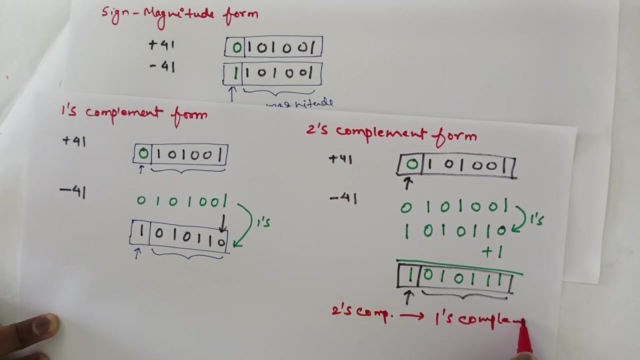 So this is the representation of the minus 41 in two's complement form. This is the sign bit and this is magnitude. We can say: two's complement of any number is one's complement plus 1.. We find one's complement And then plus 1.. So this is the representation of positive numbers and negative number in 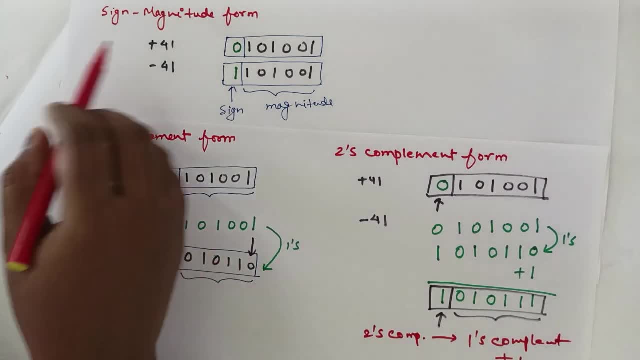 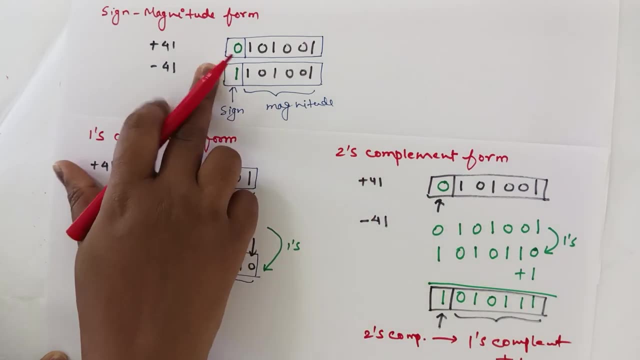 two's complement. So we can see all three sign magnitude form, one's complement form and two's complement form. Positive number representation will be same. We simply add 0 for the sign bit here in front of the number For writing the negative number methods are: 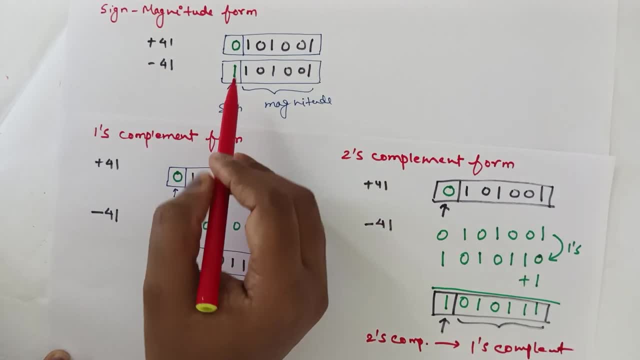 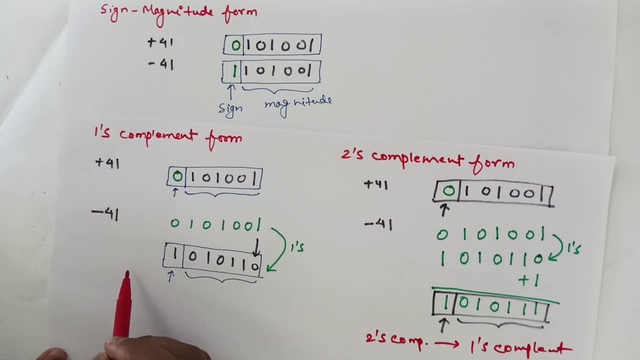 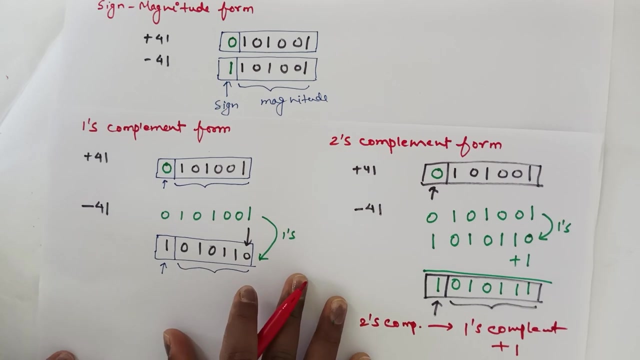 different for all these three methods. So for the sign magnitude we simply add 1 for negative number in front of the number, and for one's complement we find the one's complement of the positive number to represent the negative. And for two's complement, first we find one's complement and then add pen. 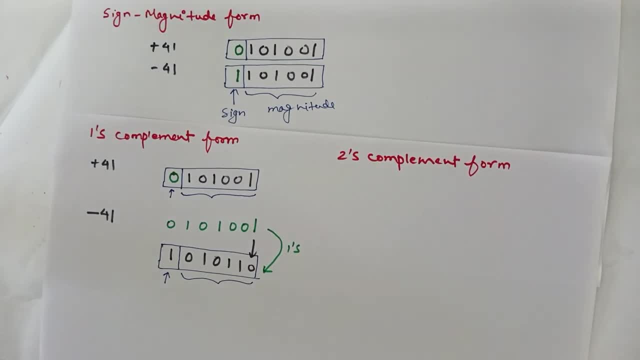 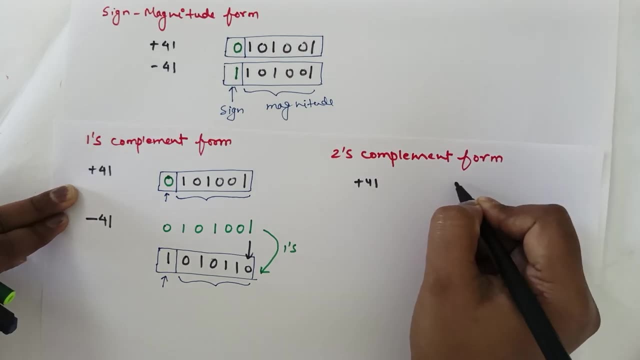 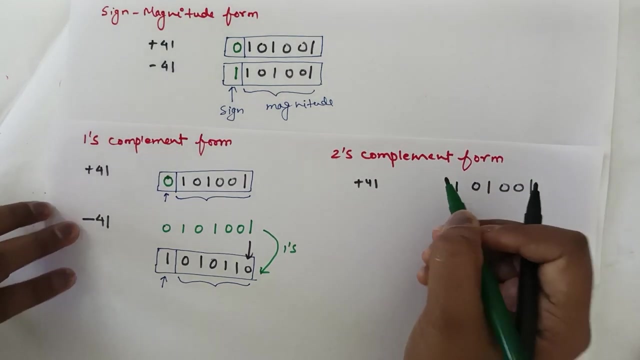 complement form. Now we will see in two's complement form We see the same example for plus 41. It will be same: 1, 0, 1, 0, 0, 1. We add a sign bit in front of the number 0, 0 for. 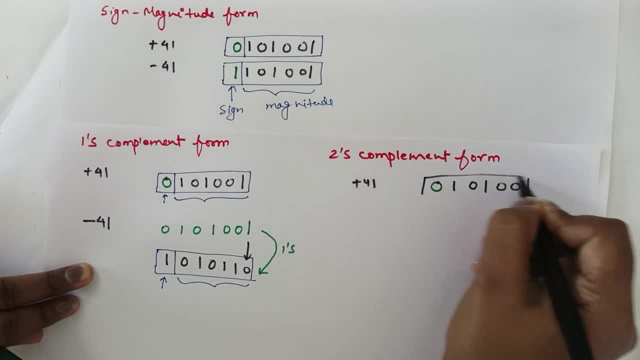 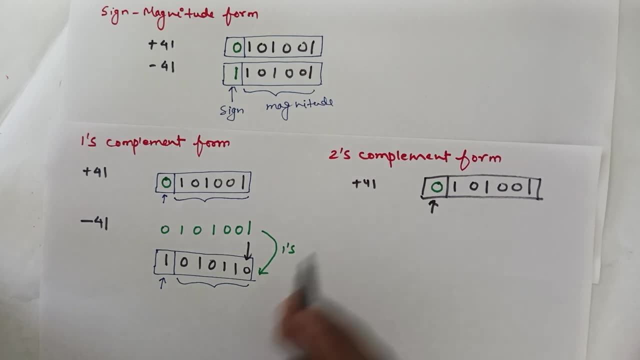 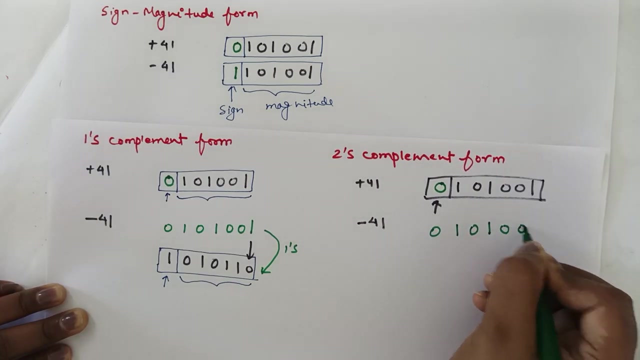 plus sign. This is sign bit, and for minus 41, we find the one's complement plus 1.. That will be minus 41.. Now we will be giving two's complement. This is 0, 1, 0, 1, 0, 0, 1.. First, find one's complement. 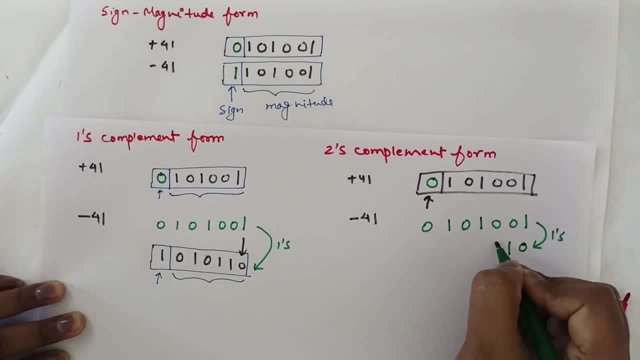 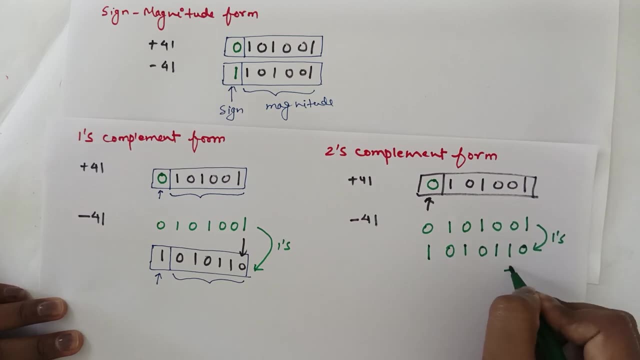 0, 1, 1, 0, 1, 0, 1.. And then plus 1.. So this will give 1, 1, 1, 0, 1, 0, 1.. 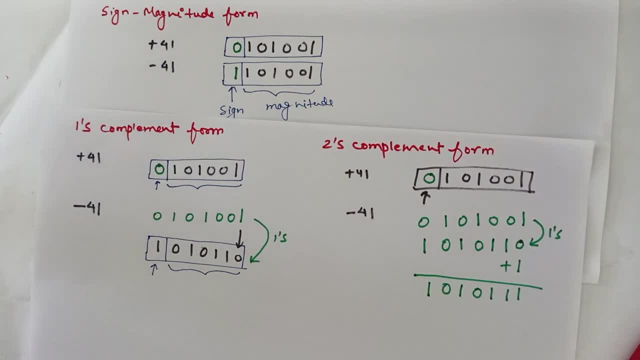 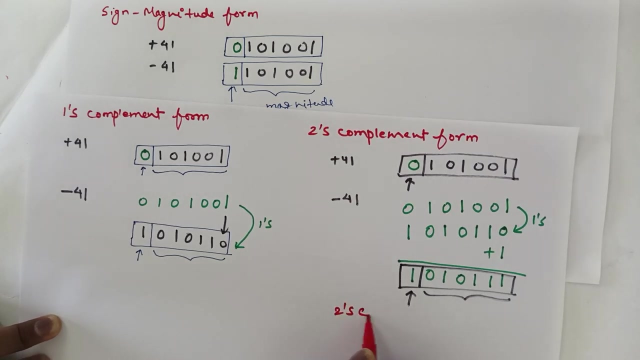 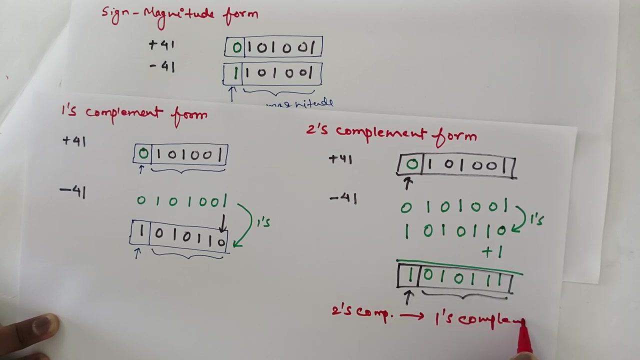 So this is the representation of the minus 41 in two's complement form. This is the sign bit and this is magnitude. We can say: two's complement of any number is one's complement plus 1.. We find one's complement And then plus 1.. So this is the representation of positive numbers and negative number in 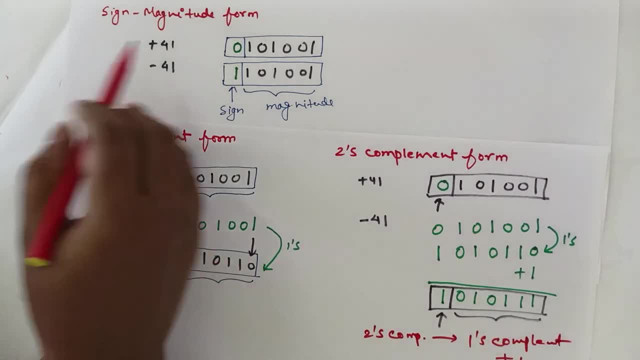 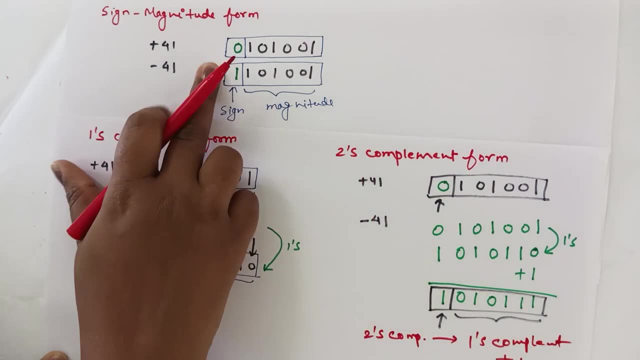 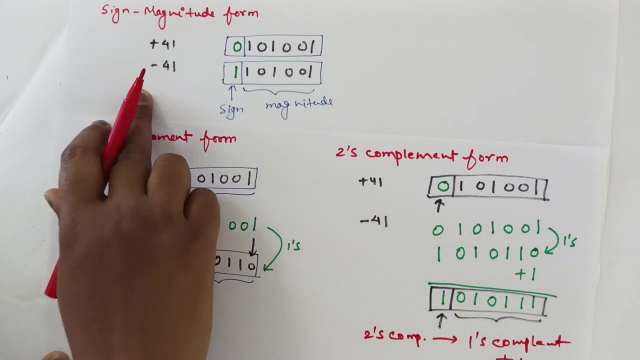 two's complement. So we can see all three sign magnitude form, one's complement form and two's complement form. Positive number representation will be same. We simply add 0 for the sign bit here in front of the number For writing the negative number methods are: 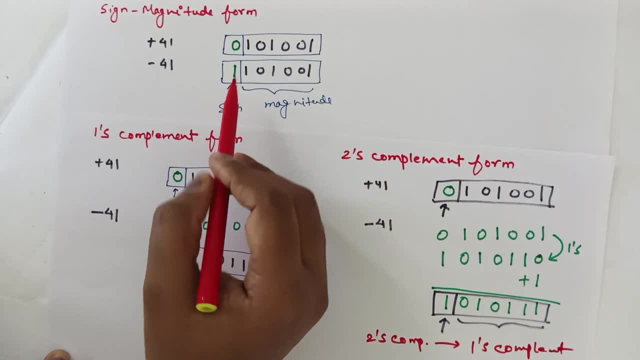 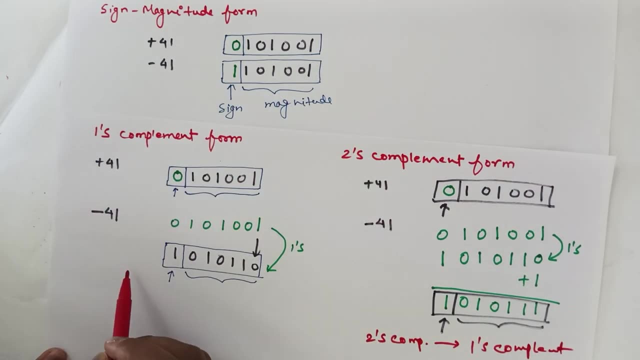 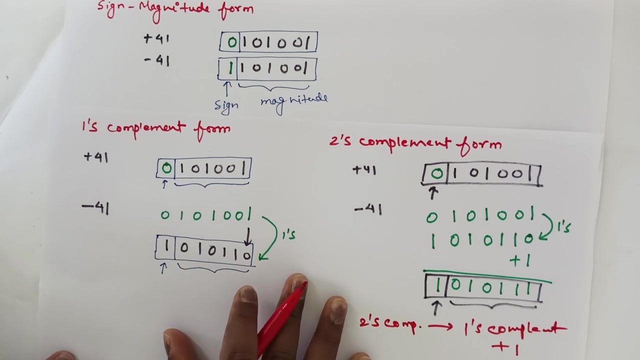 different for all these three methods. For the sign magnitude, we simply add 1. for negative number in front of the number. And for one's complement, we find the one's complement of positive number to represent the negative number. And for two's complement, first we find the one's complement and then add 1 to. 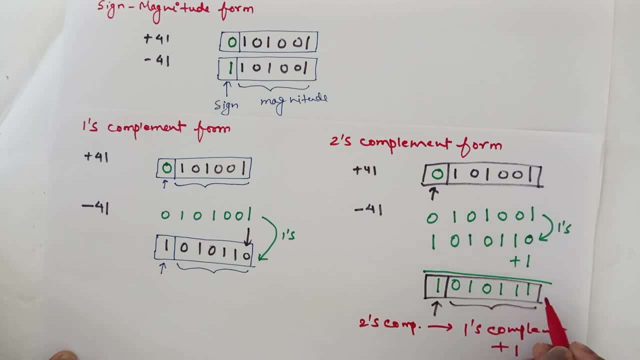 find the two's complement. That will be the negative number representation in form of two's complement. Thank you.